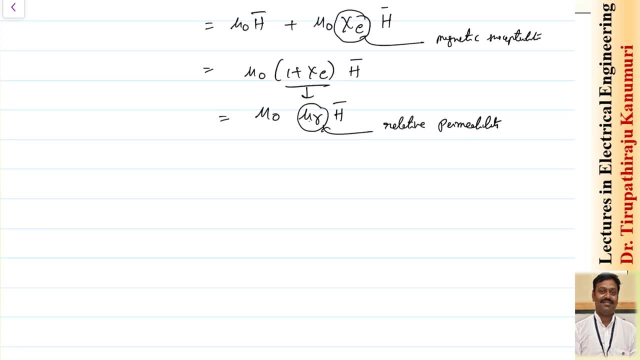 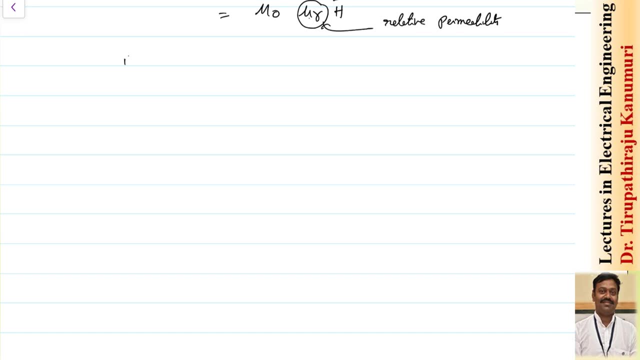 the depend when it is exposed to the external field or when the external field is applied around the material. there are basically three different broad categories of the materials. so first one is called as the dia magnetic material and the second one is called as the paramagnetic material and the third one is called as the ferromagnetic materials. there are 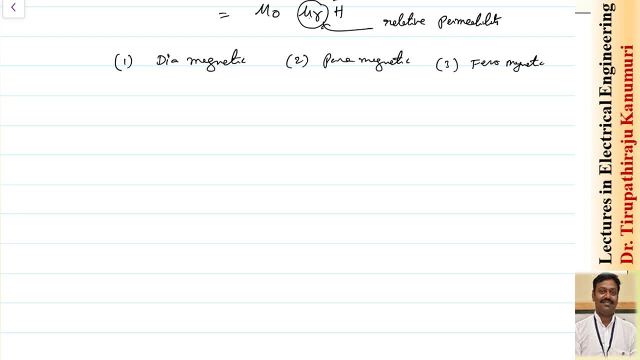 some more other materials, but these three are the most broad way we can divide the magnetic materials. let us take each one of them in detail. so first i am starting with dia magnetic materials. so first i am starting with the dia magnetic material, the, this dia magnetic material. because this magnetic material? due to, because we have 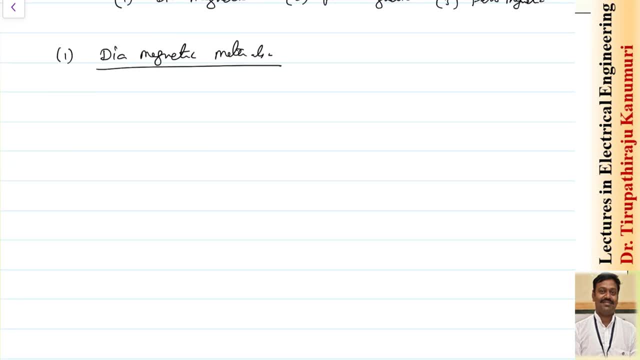 seen that, how this magnetization or the magnetic dipole is coming. so if you take any atom we have shown the central nucleus will be there around that, the electron will be orbiting around its own axis, which is called as spinning of the electrons, and second one, the electron orbits. 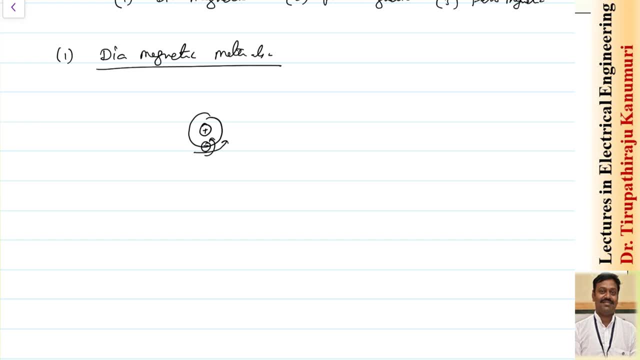 around the nucleus also. so there will be two times of magnetic moments we have seen there. one is because of spinning and second one is due to orbiting. in this type of magnetic materials the electron spin will be equal and opposite to magnetic moment due to orbital electrons. that 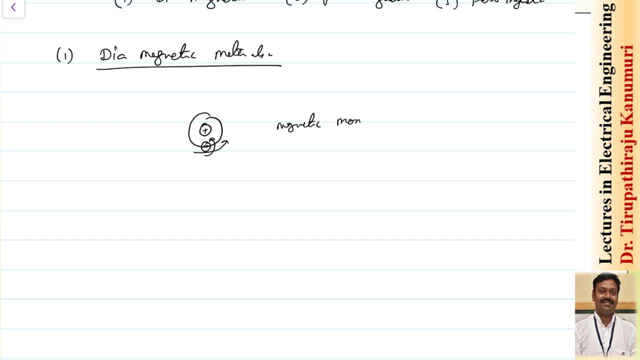 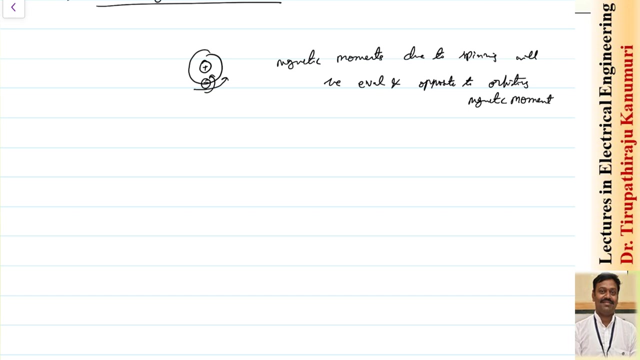 means the magnetic moment due to spinning will be equal and opposite to orbiting magnetic moment or the magnetic moment due to orbiting electrons. so here i am writing on a glass screen. that's why handwriting doesn't come properly. please try to understand the concept. i will upload the complete handwritten material in the description of this. 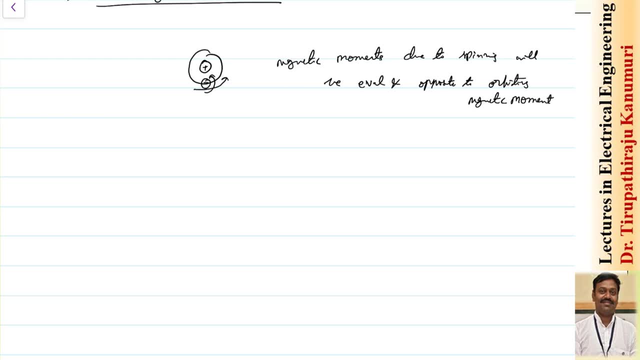 video. i will provide the link. you can please download from there. here you try to understand the concept because in theory, if you read you cannot get it properly. so these two magnetic moments will cancel with each other. so we can tell: the net magnetic moment is equal to 0 or the 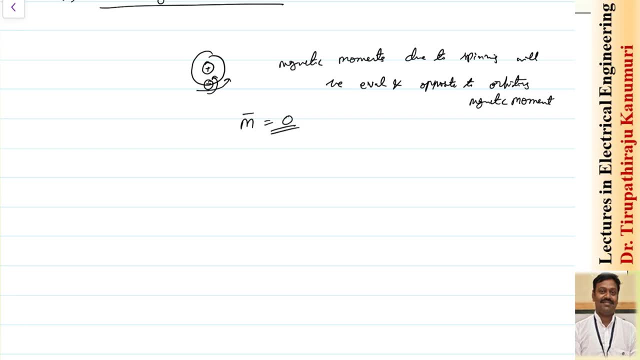 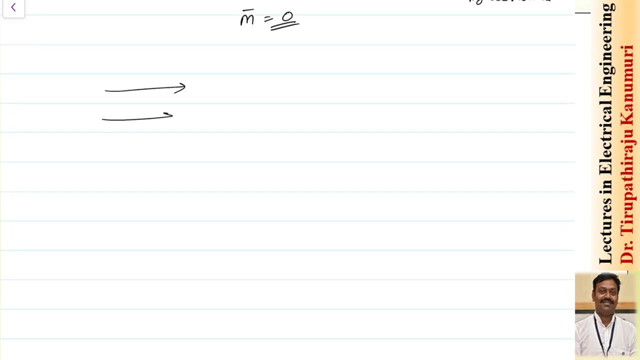 magnetization vector for this material, so that magnetization vector will be equal to 0, net effect will be equal to 0. now, when this dia magnetic material is coming from the magnetic moment it is, material is exposed to the external field. let us assume i am applying some external field. 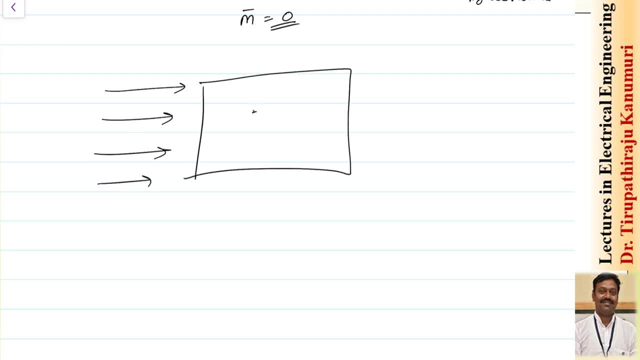 and the dia magnetic material is kept there. now what happens if we take any atom? because we know this atom will have the nucleus around that the electrons are orbiting. one is the spinning of the electrons around its own axis and orbiting. so it is observed practically that the velocity of this orbiting electrons, that means the velocity, will change. 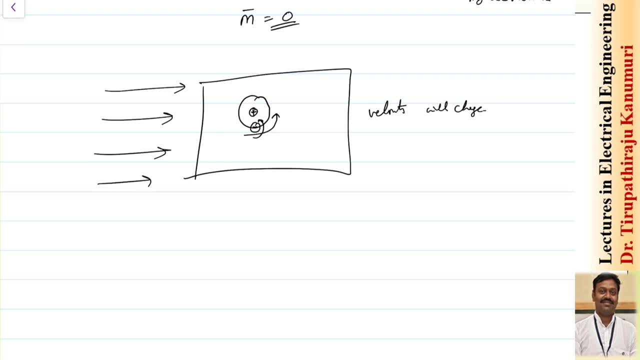 when it is exposed to the external magnetic field, because this is due to the electromagnetic term, the energy of the electrons will change as a result to the magnetic moment. the magnetic moment will be equal to 0 in the external field because this is due to the electromagneticثal field. 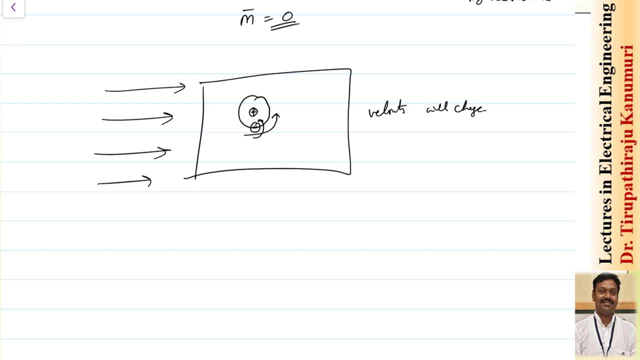 that experiences on this, or the torque experienced by this moving or the revolving electrons. so now, as a velocity is changed so automatically that net magnetic movement will not be equal to zero and it is observed that the magnetic field that is induced inside, or the m, will be in such a way. 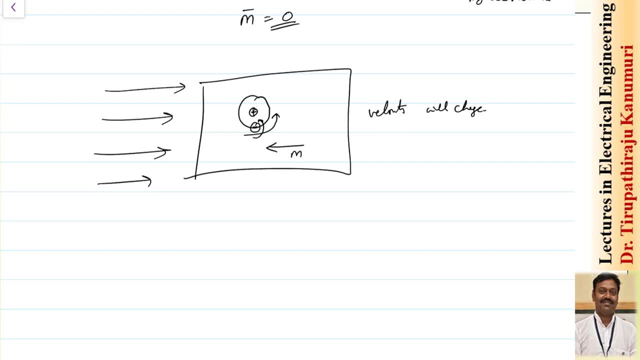 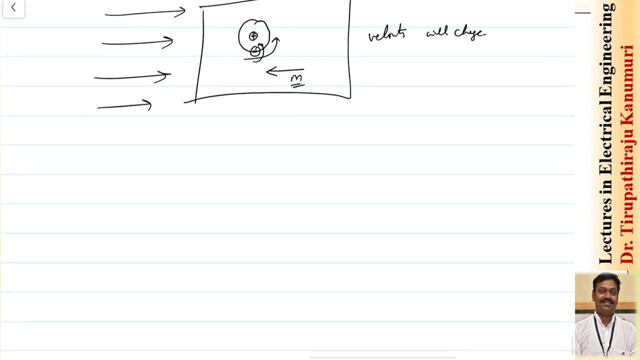 that it will be in opposite direction to the applied field. that means the m will be in the opposite direction, but practically it is observed that this value is very less. so practically this m is in opposite direction, or this i can represent as the susceptibility. susceptibility is how the 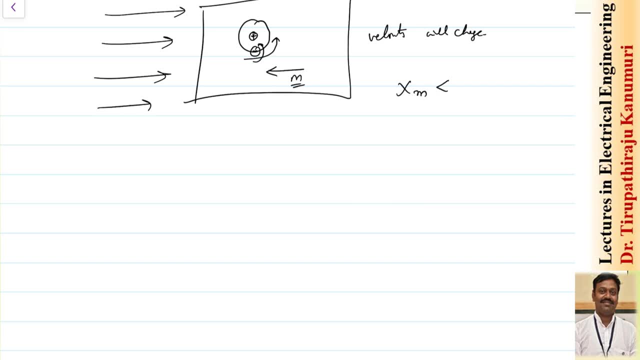 material is susceptible to the external field. it is an opposite direction. so i can take it as: m is less than 0 and the value of the relative permittivity is a permeability which is equal to muNOT, that mu multiplied by muNOT. so this will be less than or equal to 1.0. it is less than one. 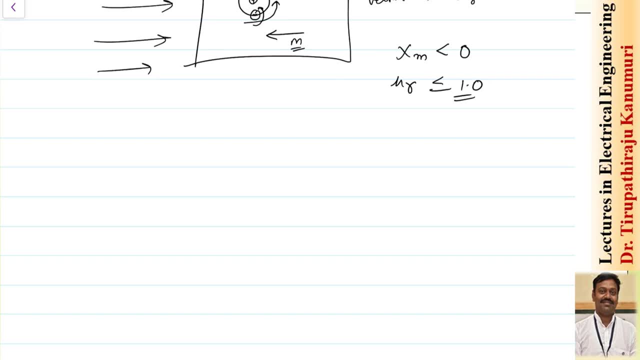 so practically, it is observed that this value will be less than in the fraction of 10 to the power of minus three to ten. Henry Sabler's symbol showing inimitableเขeyam was thinking that the właścivet value des d really makes sense. so x should be this circuit when you are talking about in terms of. 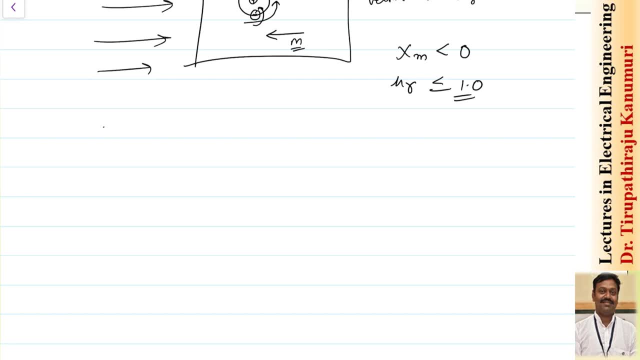 10 to the power of minus 5, but in the negative side. so the example of such materials are: the first one is the copper. so the copper, the value of chi m, is observed as 0.95 into 10 to the power of minus 5. similar is the case gold, silver, lead, silicon, diamond, bismuth, antimony, mercury, zinc. 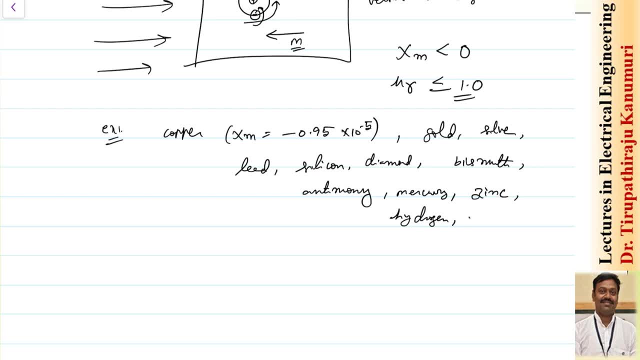 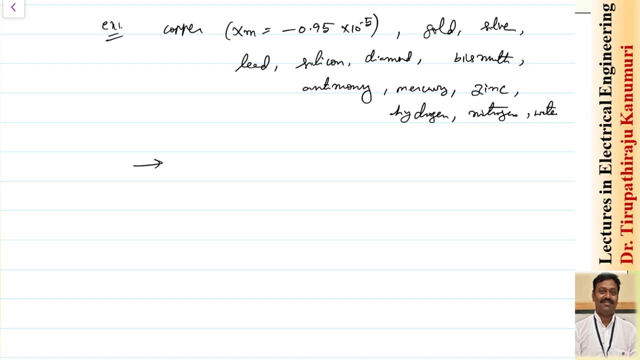 hydrogen, nitrogen, water, etc. these type of material comes in this type of property, they exhibit the similar type of property and it is also observed that there will be linear relationship between the h and the b. that means these materials can be called as linear magnetic materials. linear magnetic material. 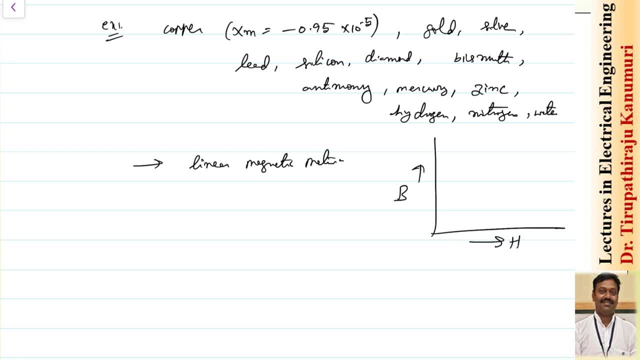 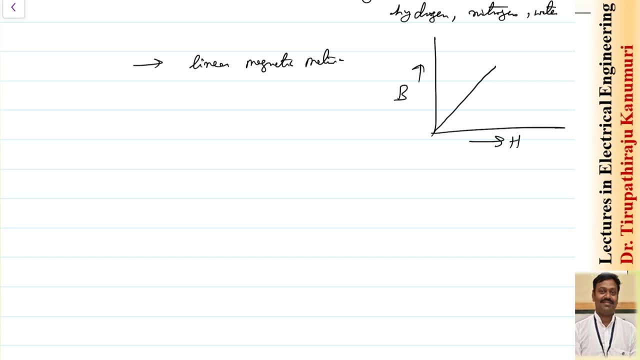 in the sense when i am varying the value of h, it is observed the value of the b will vary linearly with respect to changing this. that is the property of this diamagnetic materials. okay, why they are called as a diamagnetic materials? that doubts, you should get it. they are called as diamagnetic material because that. 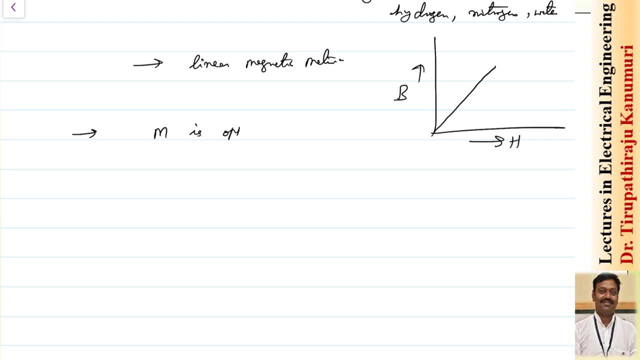 magnetization vector, this will is in opposite to h, because that m will be opposite to h as it is opposite to h. so that's why it is called as the diamagnetic. the reason why it is called as dia is because it is in the opposite direction. so now, when you bring the diamagnetic material near to, 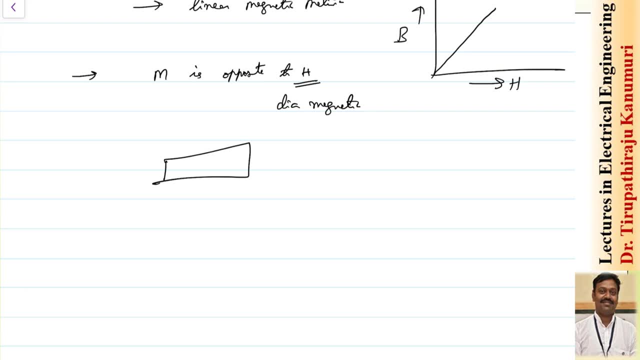 some permanent magnet. let us assume i am taking a bar magnet. so for this bar magnet i have to bring a diamagnetic material. so there will be a repulsive force on the diamagnetic material, because why? the m that is produced will be in the opposite direction, or we can tell that there will. 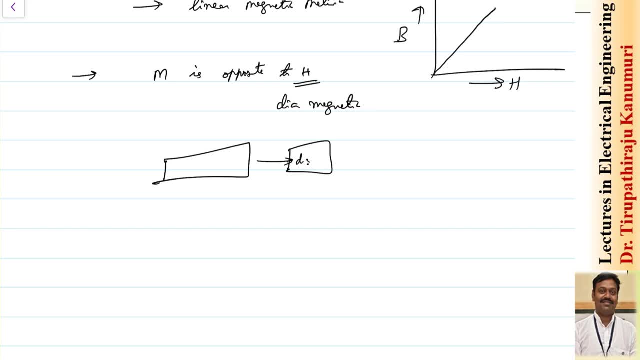 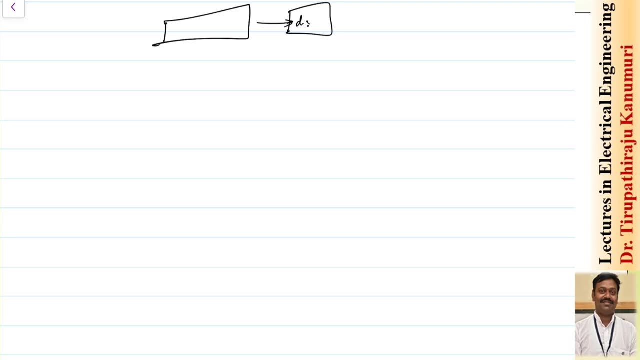 be a repulsive force when the diamagnetic material is brought near to a bar magnet. this is about diamagnetic material here. i am not writing the theory. you can please refer to my material and download from there here i want to only explain the concept because i want to teach in minimum. 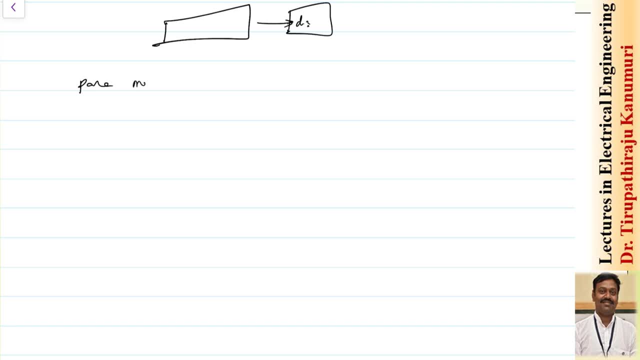 possible time. and now going to the next type of material, that is, paramagnetic material. that is paramagnetic material. so this paramagnetic material, the value of the chi m, or the relative permeability that will be the chi m or susceptibility, is greater than zero and the 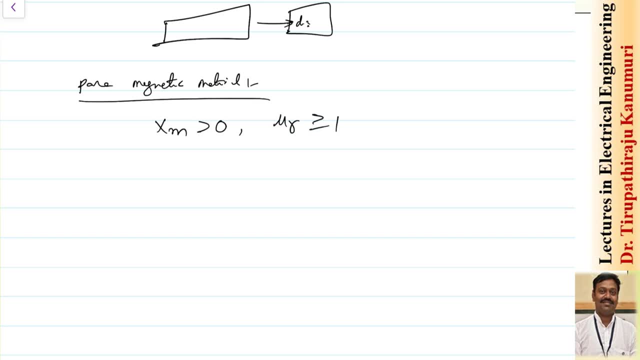 relative permeability will be greater than or equal to one and this value of chi m, this also will be very less but positive. it will be in the order of 10 to the power of minus 5 to 10 to the power of minus 3, but in this material it is positive. so in this magnetic materials, whenever 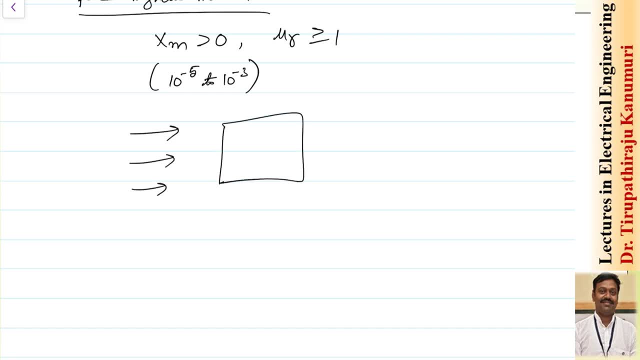 the material is kept in the opposite direction, it will be in the opposite direction, so this will be in the same direction and parallel to this applied field. so, as it is parallel to the applied field, that's why it is called as paramagnetic materials. the name came because they align in. 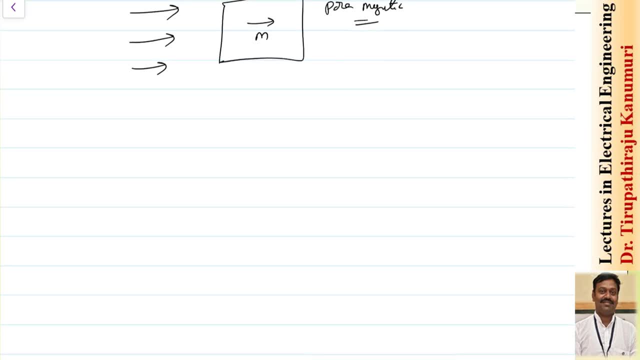 the same direction, but the effect of magnetization will be very less. that means they have very less or weak permanent magnetic movements or this orbiting and the spin movements does not cancel out in this type of materials and generally they are randomly aligned. so when the external magnetic field is not there it will act as a normal material only. but when the external 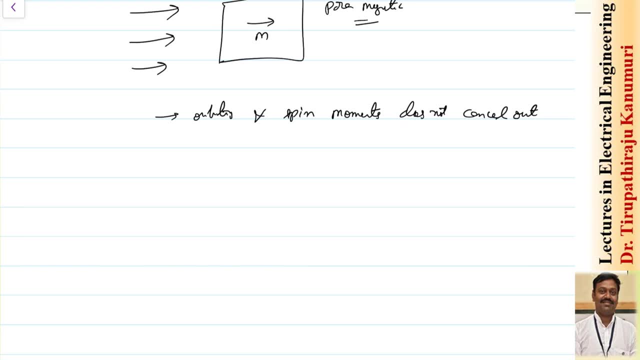 field is applied. this: whatever this small magnetic moment is there, that magnetic moment, that magnetic materials or the dipoles will align in the direction of the external magnetic field, so it will start acting as a magnet but has the minimum value of the magnetic field. so this is the magnetic field. 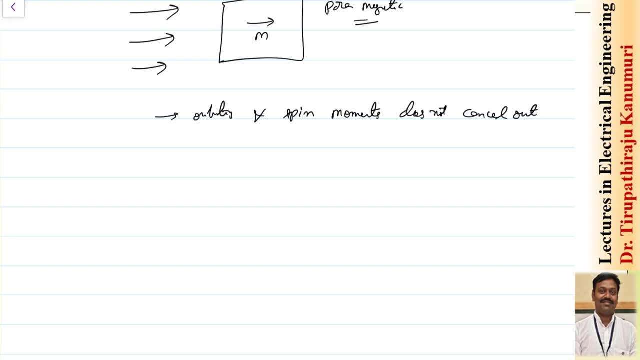 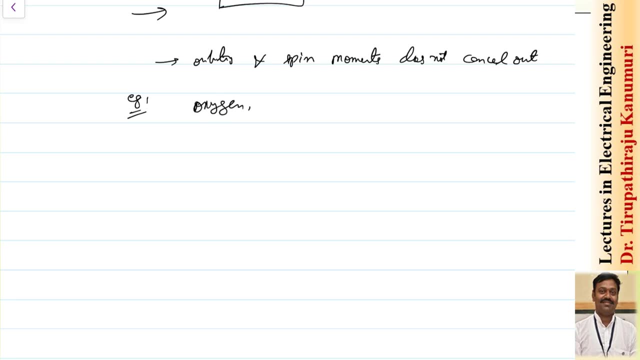 of the attractive force it will have the very weak attract to force and the second one. this example of the materials that we go through. the example is oxygen is one type of material, then platinum, tungsten, potassium, aluminum, chromium, manganese, etc. these are some of the materials which comes under the paramagnetic materials. 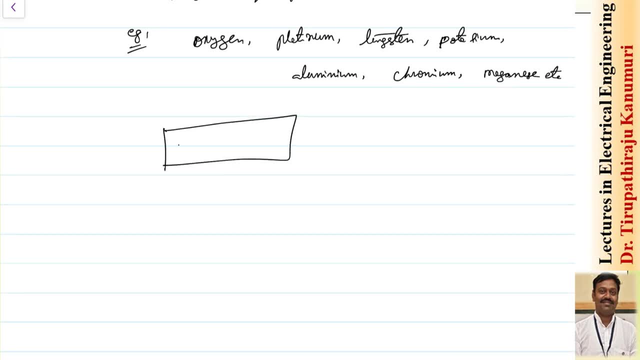 so paramagnetic material property is when you bring it near to a bar magnet. so if you bring the material near to the bar magnet, that material will be attracted towards the bar magnet. there will be attractive force. but in this type of materials generally the effect is very less. 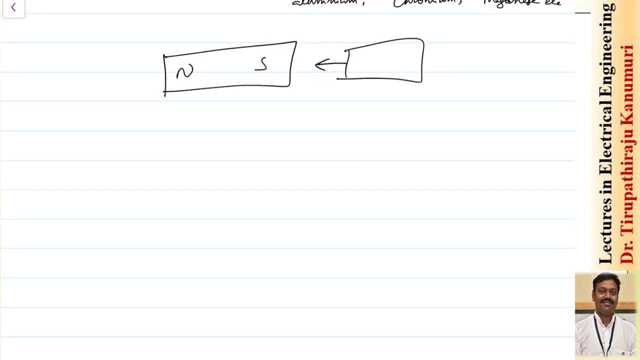 and this material has one more property. this material depends on the property, depends on the temperature also. so if the temperature is increasing, so automatically the value of the paramagnetism or we can tell that the magnetization effect will be decreased and it will directly convert to completely convert to diamagnetic material if the temperature is crossed beyond. 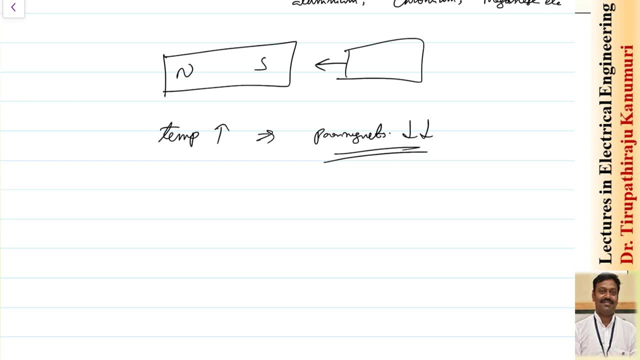 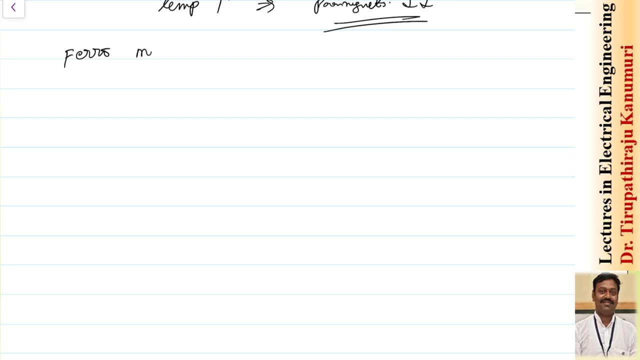 some limit. generally that temperature is called as curie temperature. so that thing you have to observe from here. so now let us go to the main type of material that is used in practice, that is, ferromagnetic materials. so in the ferromagnetic materials these are nothing but the paramagnetic materials. but 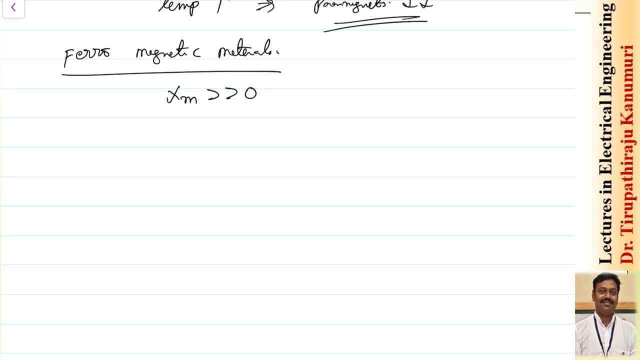 the value of the chi m, or the susceptibility, will be far, far greater than zero, and the value of a relative permeability is far, far greater than one. the example of this one is iron, nickel, cobalt and the other alloys which are made up of these materials, and the their alloys, the cobalt. 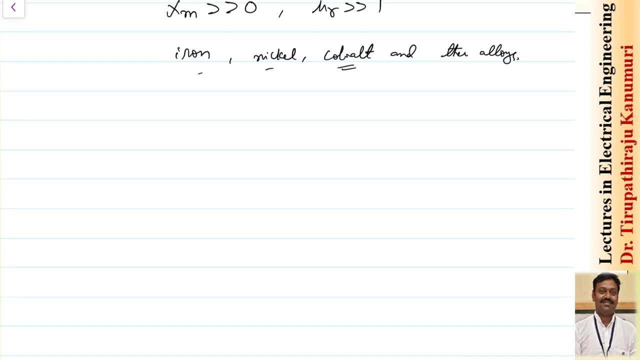 materials and the other alloys which are made up of these materials and their alloys, the cobalt, nickel and iron. they are made with combination of these things. so in this type of materials, the permanent, there will be strong, permanent magnetic moments, because the more the magnetic movement, the 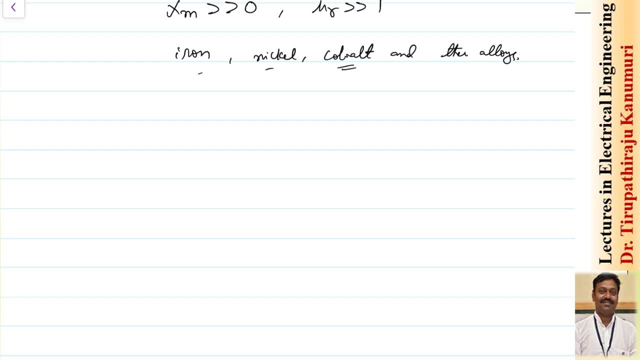 spinning and the orbiting magnetic movements will not cancel out. so the permanent magnetic movements will be there and this permanent magnetic movements also. if you take the material in the microscopic level, so that material can be divided into different type of domains, so a domain is the smallest possible particle where the dipoles are generally distributed in groups. 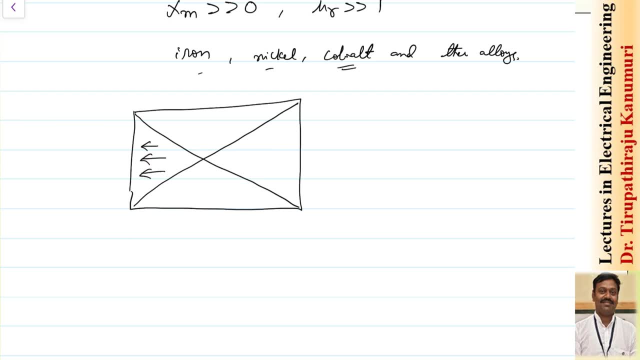 is the smallest possible particle where the dipoles are generally distributed in groups. that means a- let us assume a group of the dipoles are around like this, so this we call as one domain. in the neighboring domain, again, group of the particles or group of the dipoles are aligned. 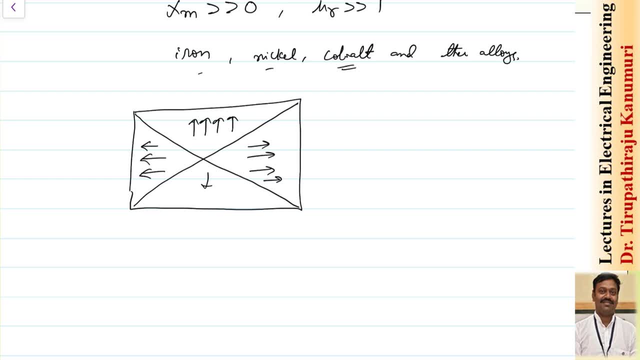 in some other direction. same thing is the case in different domains. they are randomly distributed. here i am drawing systematic, but it is not the case practically. so this: each one where a set or the neighbors are forming a group and aligning in the same direction, that is called as a domain. 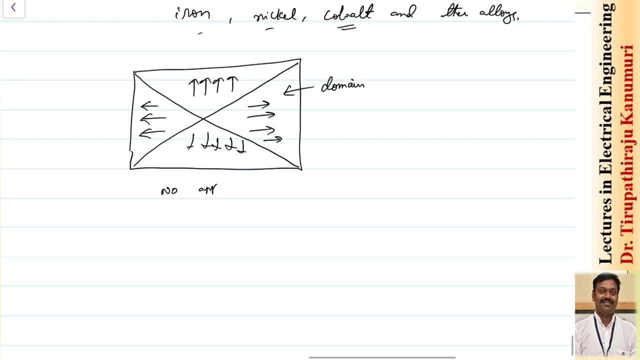 so this is the case when no applied field is there, when no applied field is there, but now, when the external magnetic field is observed, it is observed that this will, they will start aligning in the direction of the field. let us assume the field is applied like this: this is: 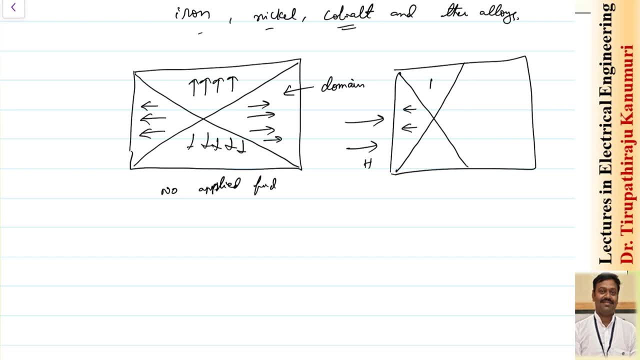 the direction of h. so now the number of elements or number of dipoles in each of this domain will goes on decreasing and they will start aligning in the direction of the magnetic field. so this is the case when you apply external field, So they will try to align in the direction as the external field goes on increasing the alignment. 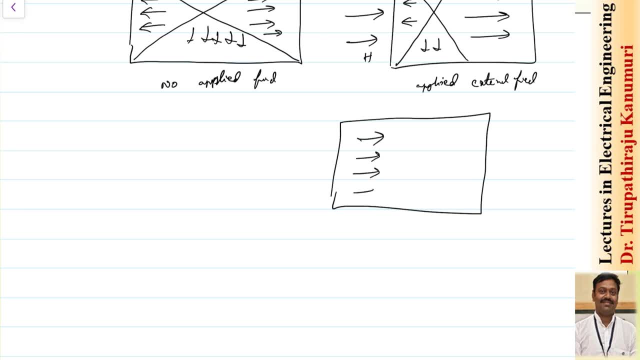 will goes on increasing and a point will reach where all your dipoles will be aligned in the direction of the magnetic field. Once they are completely aligned in the direction of the magnetic field, there is no further alignment possible or we can tell the material is completely. 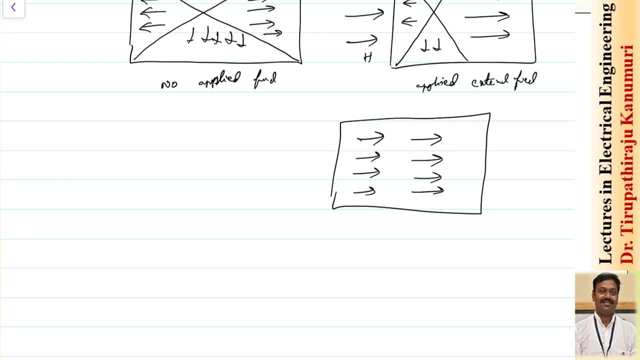 magnetized or we tell that the element is saturated, the element reaches the saturation. Above that, even if you are increasing the field, external field, it is not going to align because there are no extra atoms available or extra dipoles available to align them in the direction of the magnetic. 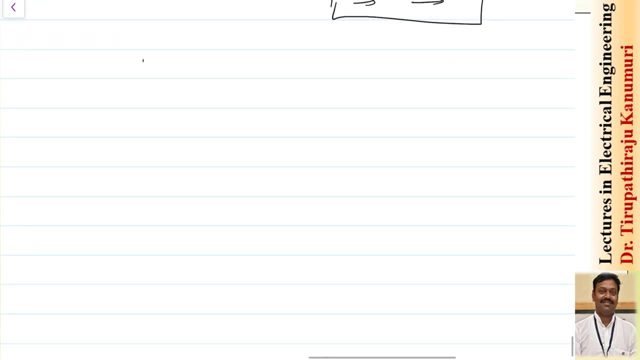 field or if you draw that practically, how the variation will be there for this type of materials. So I am taking the value of the h and how the value of the mu r is changing. It is observed the value of the mu? r is not constant in this type of materials. the relative permeability will be. 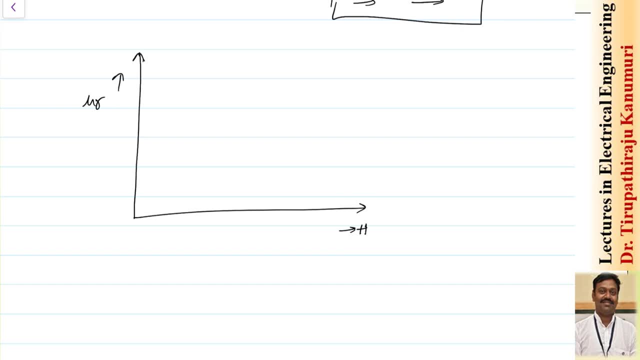 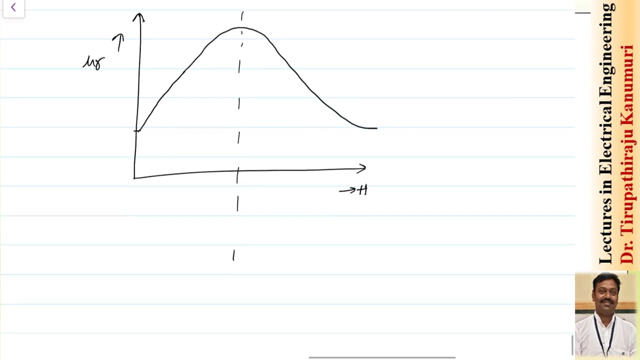 non-linear, or the chi m, That is, susceptibility, also is a non-linear. So if you draw the curve you will get. the value of mu r will be like this: It will increase up to certain extent, after that it reaches the peak, after that it will go on decaying and this will be the maximum point. So this is the value of mu r. 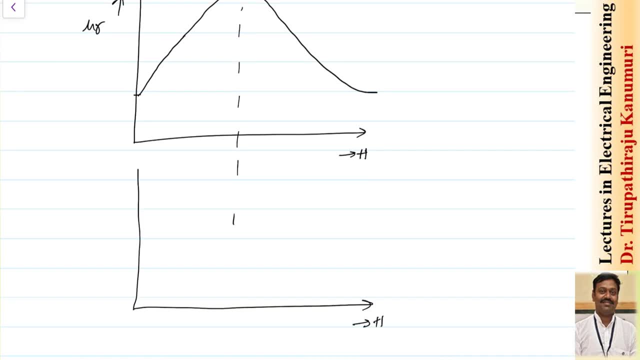 Let us try to draw what will be the value of b because of the change in the value of mu r. So this is the change in the b, how the b will change. So the b will change like that: initially: the dipole- so many dipoles are there which can be aligned. So initially, when you apply, 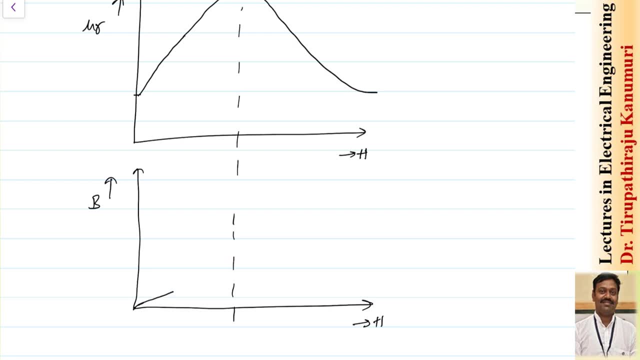 the dipole. so many dipoles are there which can be aligned. So initially, when you apply the magnetic field, they will align at a faster rate. or, as the h is increased, it will curve, will start like this: it will reach some peak and after that it will start saturating. So it will start. 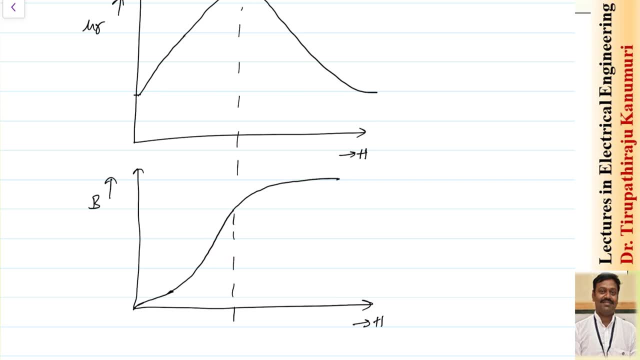 saturating Initially, some energy is required to align them in the direction. that way, the slope is not like this. the slope is less. Then it will increase at a faster rate up to this point. So we can tell this region as the second region. This is the first region. This is due to the 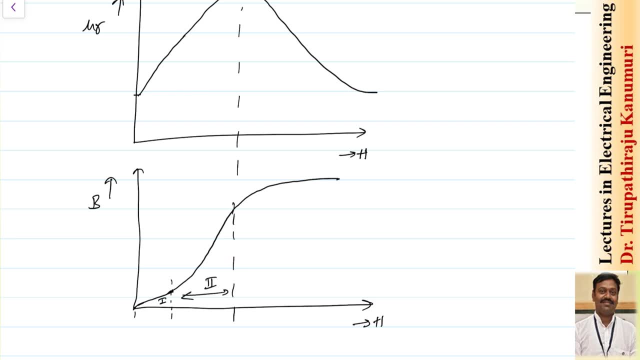 magnetic materials or any element will not try to align that much easily in any other orientation. or in order to orient their magnetic materials in a particular direction, they will need more energy because of the friction- atomic friction- that is available. That is why more h is required in this region. But after this region. 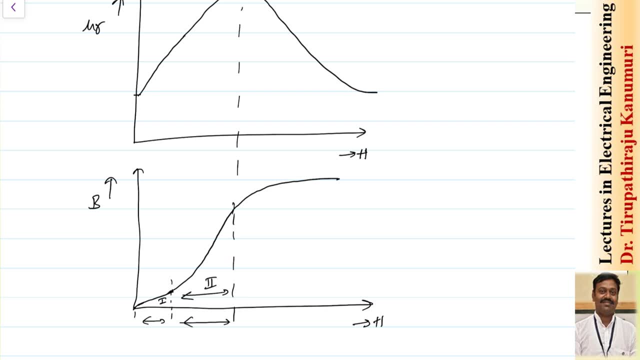 they will start aligning at a faster rate. That means for a small change in h will create more change in b. That is why the slope is at a strip. So after that a point will reach. after that it will go on going into saturation. So this region, I can draw the magnetic field. So this is the 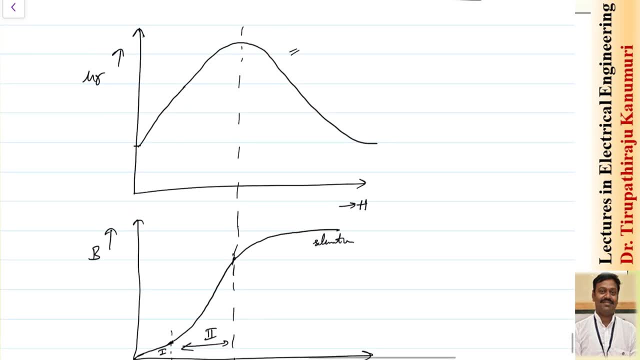 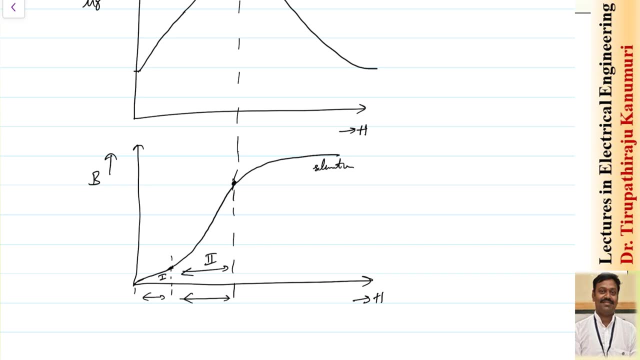 point we can call as the saturation region. So this is due to the variation of mu r, because b is nothing but mu naught mu r into h. I hope this is coming. So how to get this point where this value of mu r will be maximum? We can just draw a tangent from the origin. The tangent will touch. 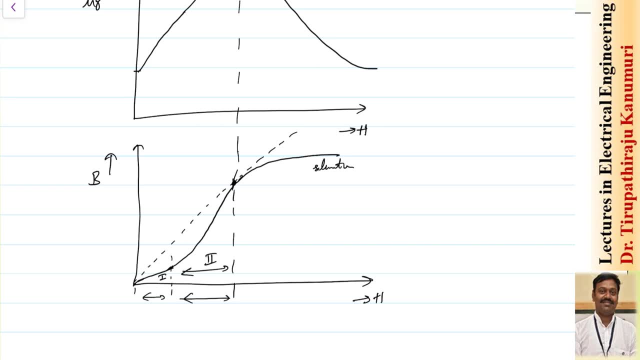 this bh curve. Wherever the tangent is coming at that point the mu r will be highest. In that way I can calculate it, because we have to take the slope of db by dh at the point any point to get the incremental permeability at that point. 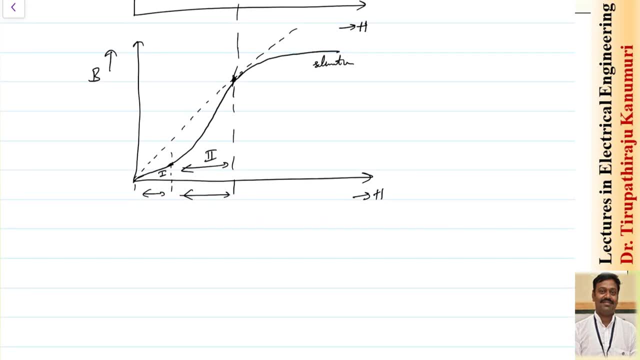 So now, coming to the characteristic of this, you can see, it is not not not a linear curve. This is the first thing you have to observe And the second one: this amount of magnetization when compared to the paramagnetic material in the ferromagnetic material, the net magnetic field. 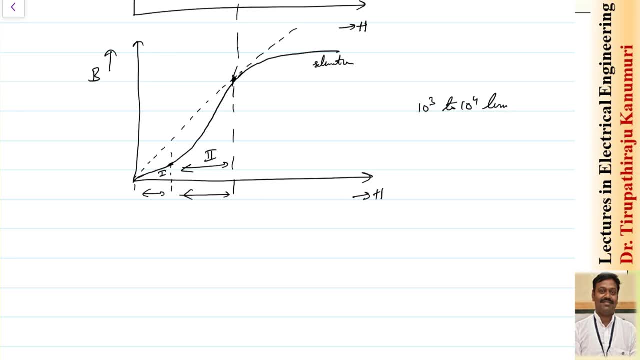 will be 10 to the power of 3 to 10 to the power of 4 times the applied field, So that much magnetic field will be there inside the material when this material is kept in the magnetic field. That is why they can act as a magnet at a easier. 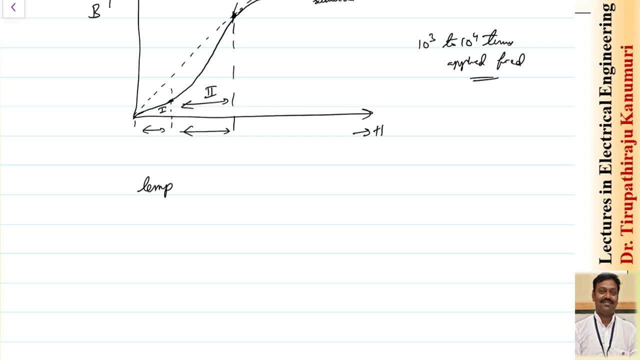 But again, these materials also. the value of the mu r or chi m depends on the temperature. As the temperature is increased, so automatically the value of the relative permeability will go on decreasing and the point will reach where the value of mu? r will be completely decreased. and it will start acting like a diamagnetic material. That means the value of mu r will approach equal to 1. So that temperature is called as the Curie temperature, and this temperature is usually nearly equal to around 700 degrees to 800 degrees for different type of materials. For iron: 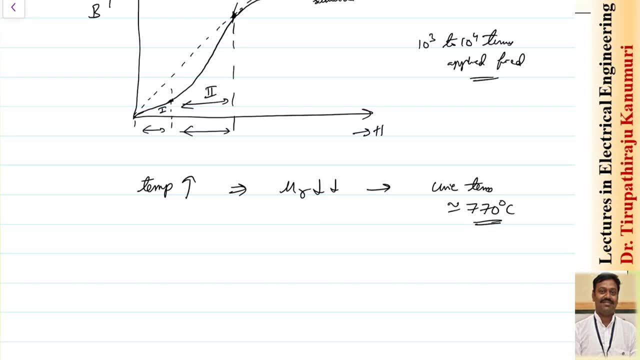 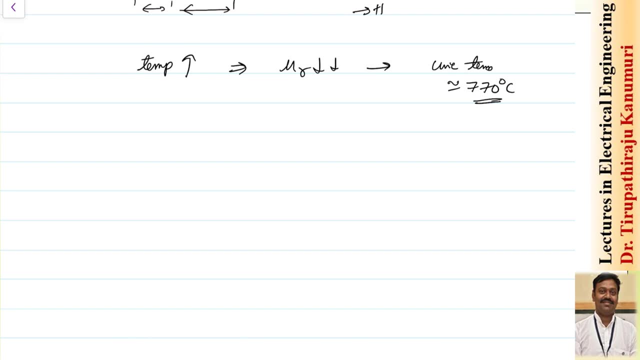 it is equal to 770 degrees centigrade, So above that it will convert as a diamagnetic material. That is the reason. if you see the fans which generally the cashiers uses in the bank, the small fans will be used. That fans the property will be. they will run for like one two hours whenever they. 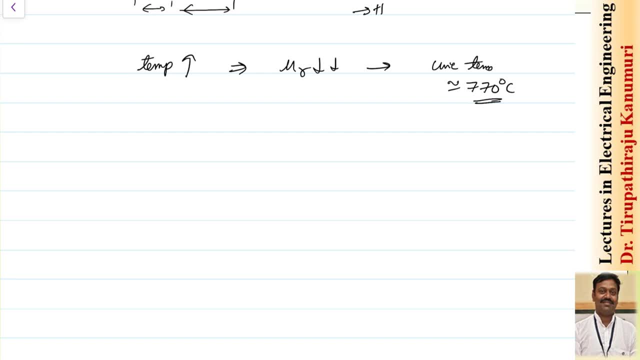 are heated up, particularly in the summer season, they will stop for some time. Again they will start automatically. So why they are stopping? Because inside there is a electric current which is electromagnetic, and when the heat is increased that material will lose its magnetic property. It. 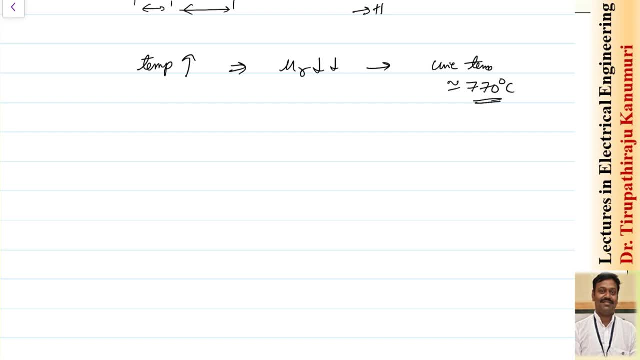 will start acting as an air core, then the required amount of flux will not be produced there, so required torque will not produce and the motor will stop. So whenever the temperature is cooled down, then again it regains its material property, then again it gets magnetized and then it will. 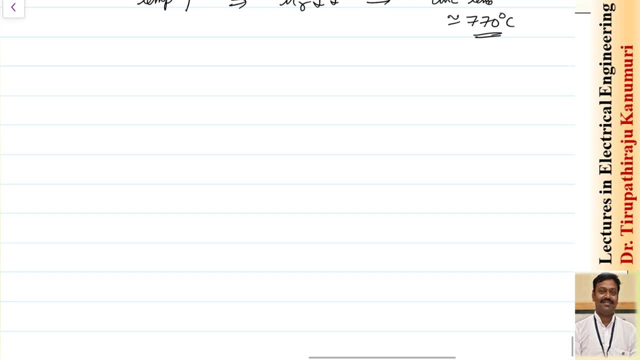 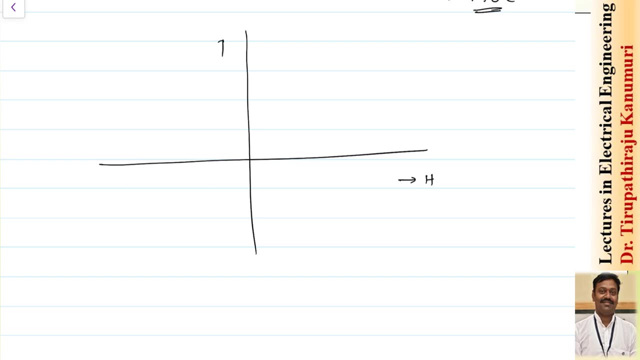 start operating in the normal way. So this is the way it is done. So now, coming to the concept, it is also observed practically when, let us take for example, initially, the material is a normal material with no previous history of the magnetization Previously it is not magnetized. So now, when you 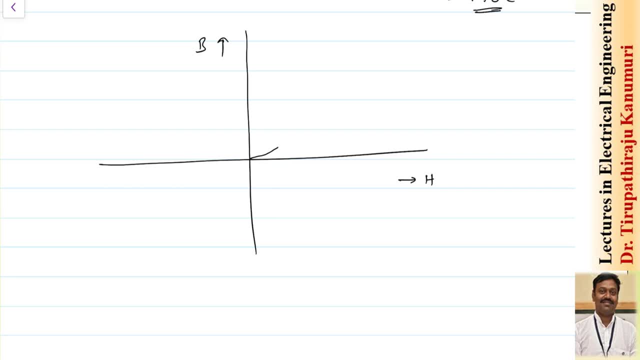 are increasing the value of the H, so it will linearly increase, like this: initially it will increase slowly, then it will increase triply, then go to the saturation. Everyone agree with me. So now, when you are decreasing the value of the H, it is observed it will not follow the same curve. it. 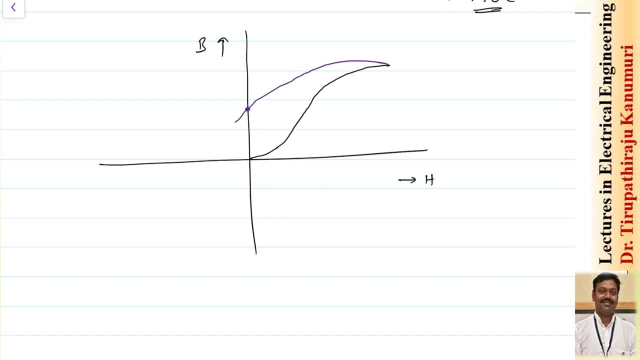 will follow some other curve and even if you make the H is equal to zero, some value of the B will still be remaining there. So this value of B that is still remaining there, This is called as the residual flux, residual flux and this property is called as retentivity. 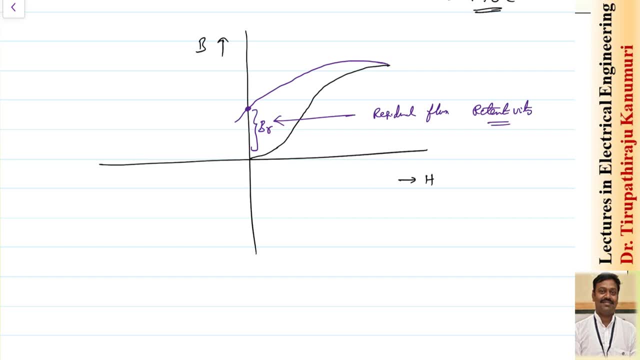 property of the material. Retentivity property means it is a property of the material to retain some magnetic field, even when the value of H is reached to zero Again. now if you want to bring the magnetic flux to zero, you have to increase the value of H in the opposite direction. So when you 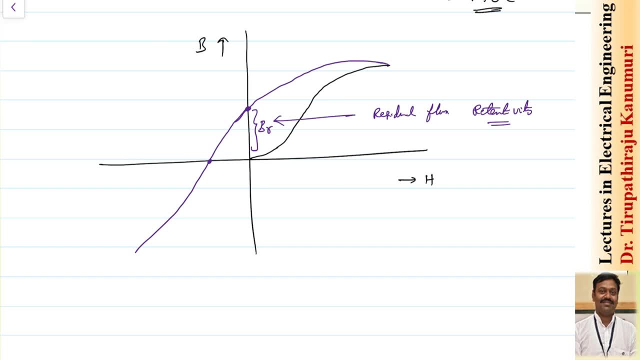 increase in the opposite direction. there is some value of the H required to make the magnetic field equal to zero. This is called as coercive property or coercivity. So this is called as coercivity of the material. So coercivity should be. it depends on the type of the material. So now it is further. 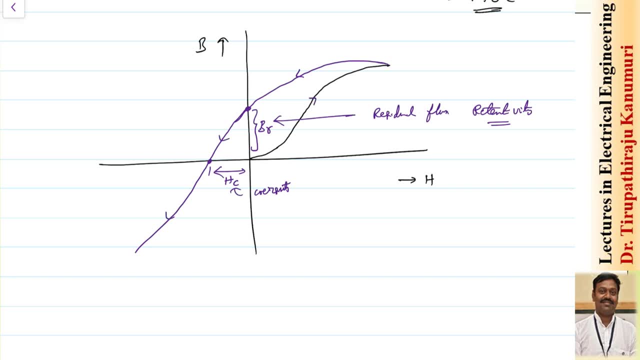 increased in the negative direction. I am just representing with an arrow. So it is following like this Again: if you are increasing it again, it will follow this path and it will reach this point. It will reach the same point. so it will follow the path like this. 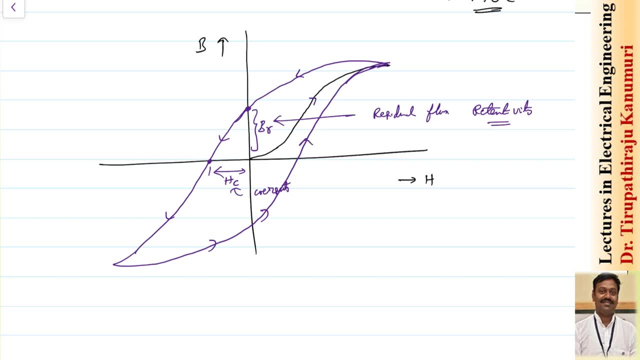 This characteristic is called as the BH characteristic curve. This characteristic is called as a BH characteristic curve. So why this BH characteristic curve is coming, Why it is not following the same path? The reason is due to molecular magnetic friction in the material, The dipoles, whenever 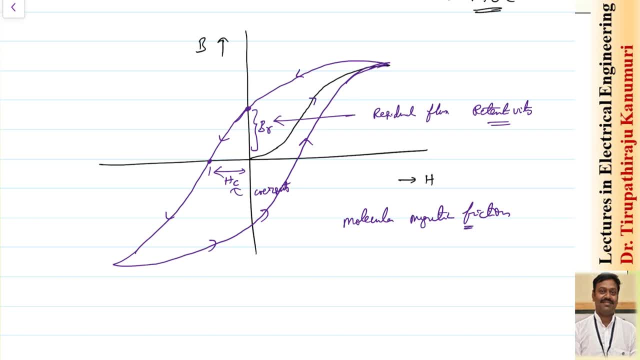 they are aligning from one direction to another direction. there will be some friction. Because of the friction, some energy will be dissipated in the form of heat. So whatever the energy will be dissipated in the form of heat will be dissipated in the form of heat. So this is called as the BH characteristic curve. 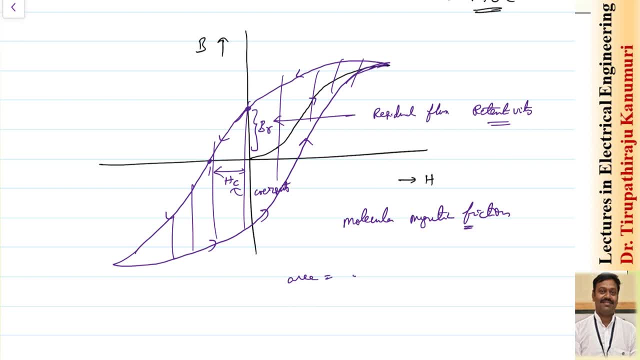 This area gives the energy loss per unit volume of material in one periodic cycle of magnetization. So if you are varying the supply like this, like if I am varying my current, like this, sinusoidally increasing up to peak, Then decreasing, making negative and bringing back to zero, So in this one cycle, this is called as one cycle of magnetization. 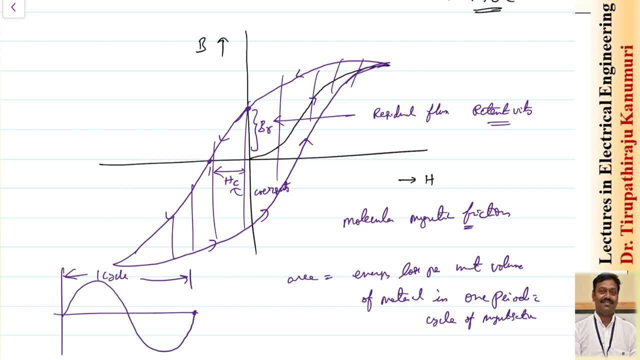 In this one cycle, how much will be the area under this curve? So that gives the energy loss per unit volume of the material. So broader the value of the BH curve, so more will be the power loss in the material. If you want to decrease the power loss- or this loss is also called as hysteresis loss, because it 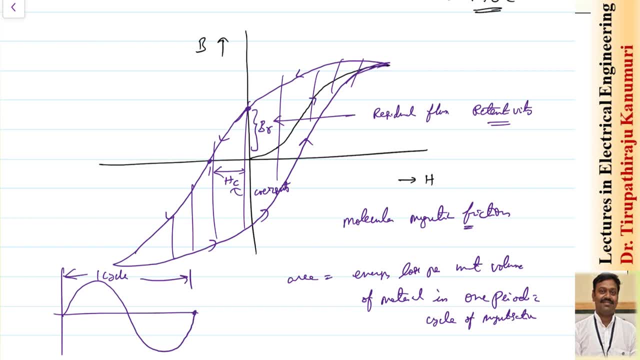 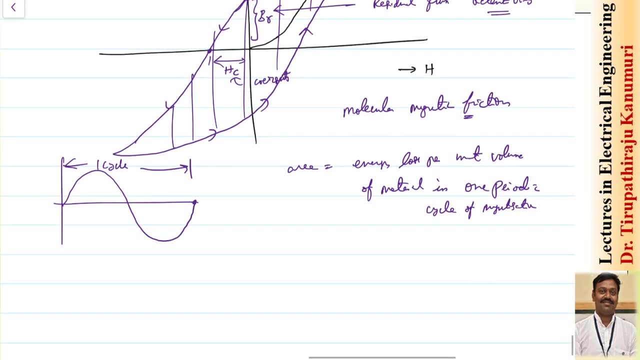 happens due to the hysteresis or the lag between the H and the B, H and B will not have the linear characteristics, So that material should have the minimum value of the curve. But if you want to manufacture a permanent magnet, that permanent magnet property should be like that: 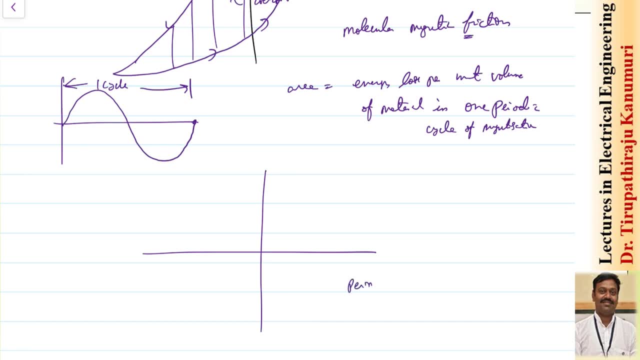 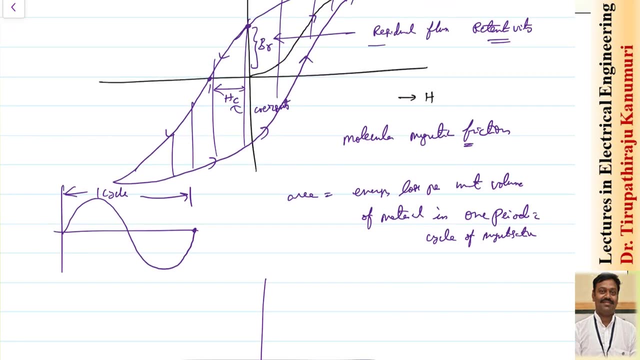 It should have the maximum value of. So if you want to make- let us assume I want to make- the permanent magnet So that mag material should have more value of retentivity, because once you magnetize and make H 0, that BR should be maximum. 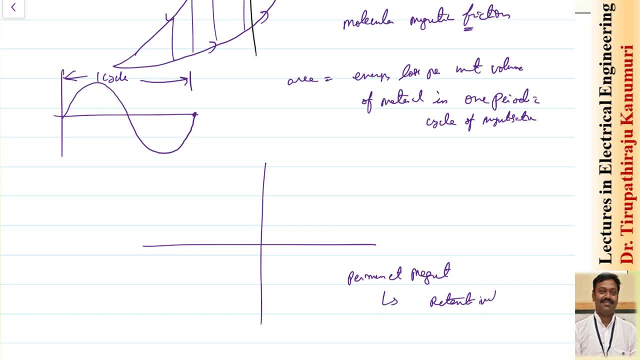 So first one is it should have the more retentivity. retentivity should be highest. and then the second one is it should have the higher value of the permanent value, etc. second one: coercivity, because it should remain as a permanent magnet even if you apply the field in.